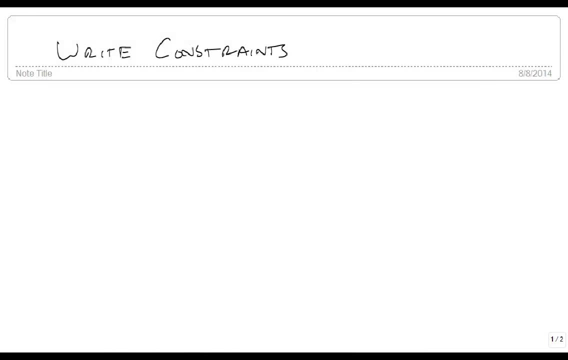 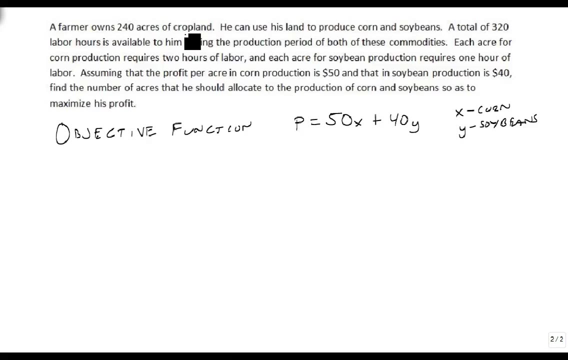 Now that we know what our objective function is, it's time to look for the constraints on the problem. So here's what we're looking at Again: farmer owning 240 acres is the same problem, but here we're going to write our constraints, And so there's a couple of